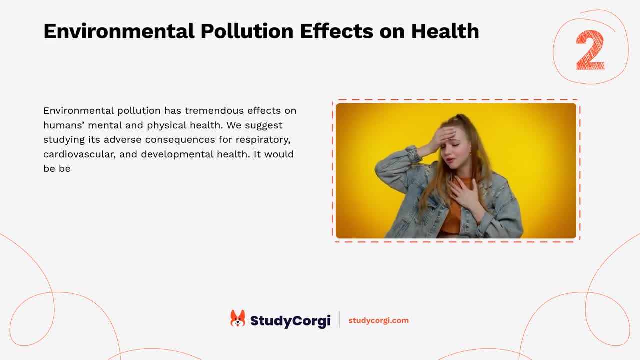 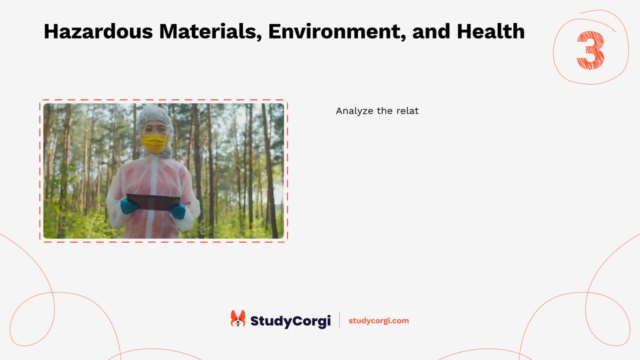 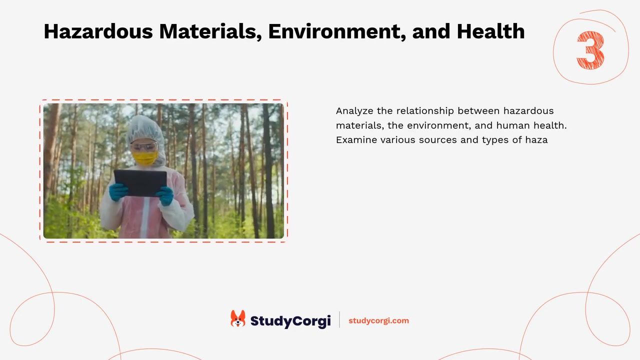 cardiovascular and developmental health. It would be beneficial to stress the significance of pollution control measures and public awareness campaigns. Hazardous Materials, Environment and Health. Analyze the relationship between hazardous materials, the environment and human health. Examine various sources and types of hazardous materials and how they impact ecosystems. and. 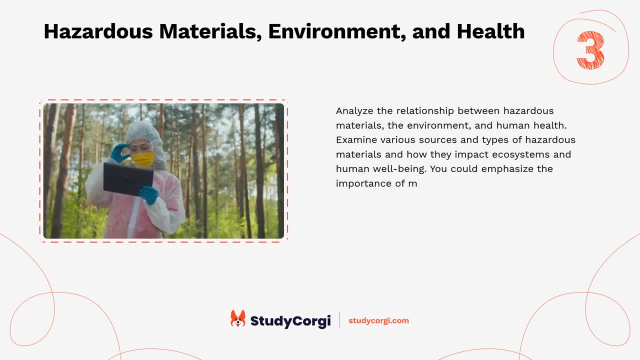 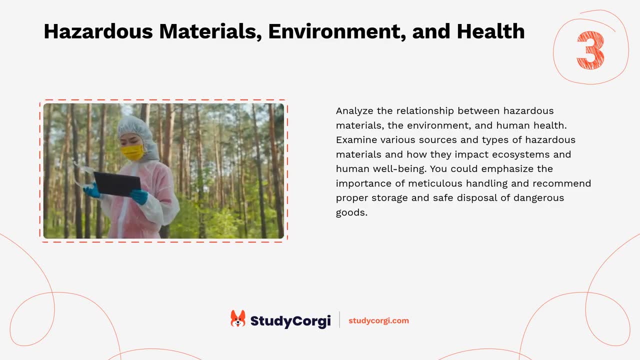 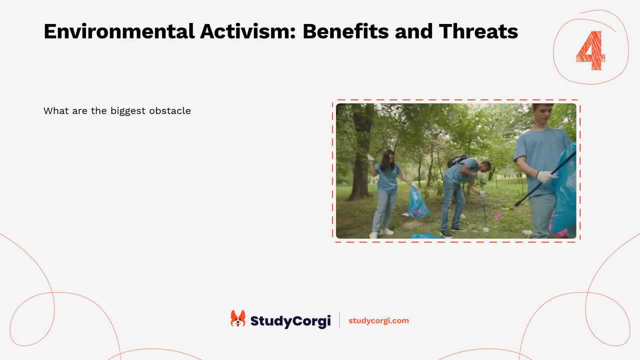 human well-being. You could emphasize the importance of meticulous handling and the importance of the use of materials that are used to control the environment, Recommend proper storage and safe disposal of dangerous goods. Environmental Activism: Benefits and Threats. What are the biggest obstacles environmental activists face? 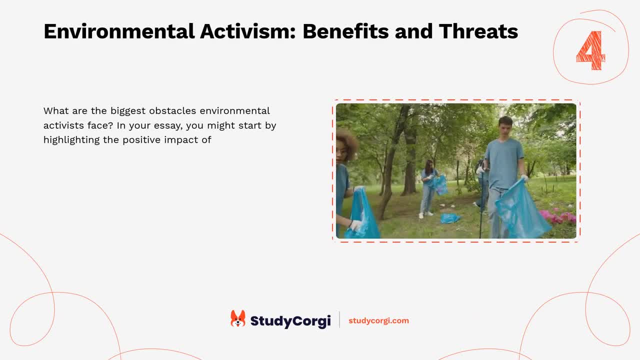 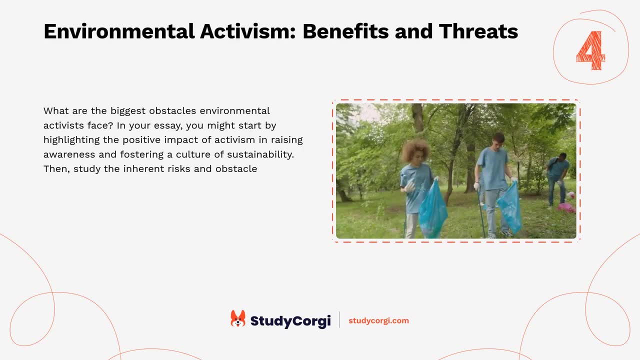 In your essay, you might start by highlighting the positive impact of activism in raising awareness and fostering a culture of sustainability, Then study the inherent risks and obstacles faced by activists, like the importance of inclusivity, collaboration and non-violent approaches. 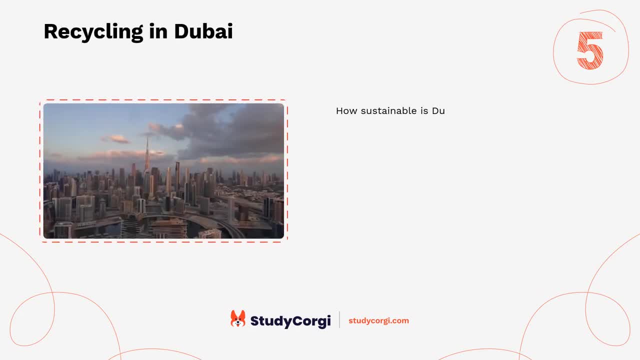 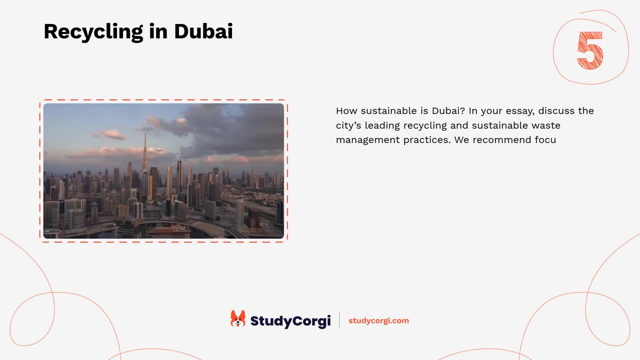 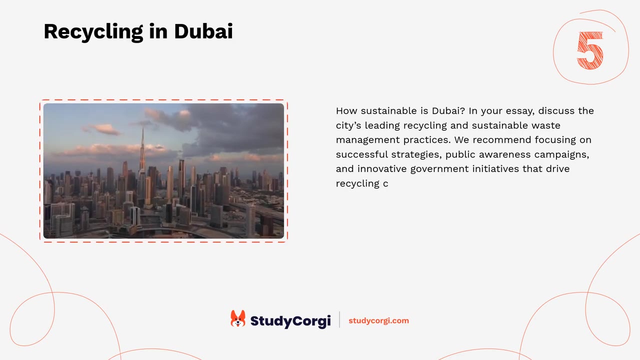 Recycling in Dubai. How sustainable is Dubai? In your essay, discuss the city's leading recycling and sustainable waste management practices. We recommend focusing on successful strategies, public awareness campaigns and innovative government initiatives that drive recycling culture in Dubai. Highlight the role of community engagement and public-private partnerships in promoting 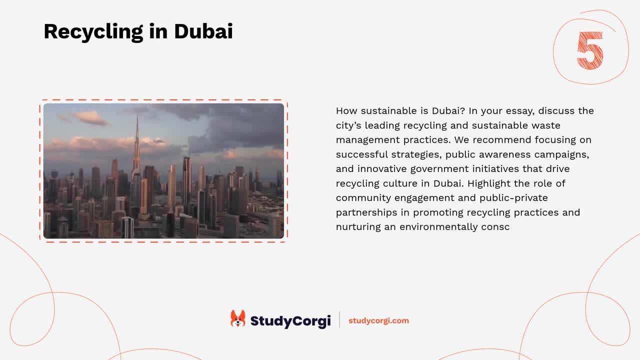 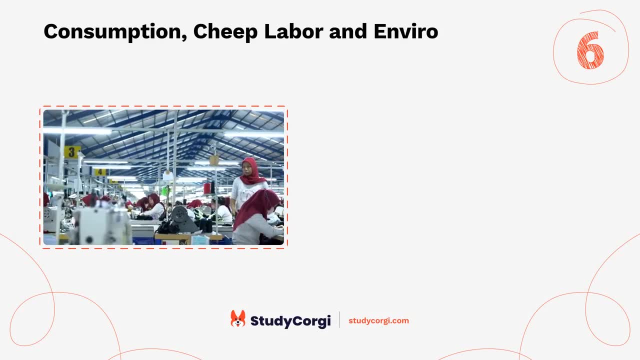 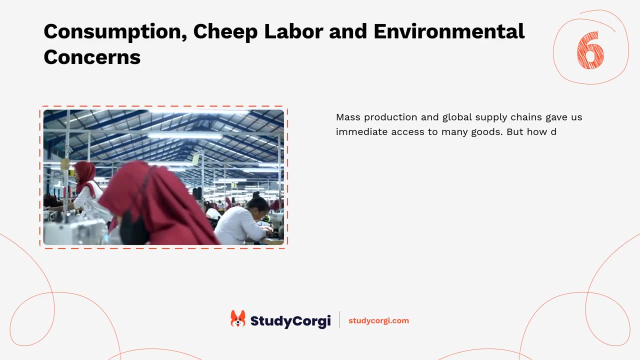 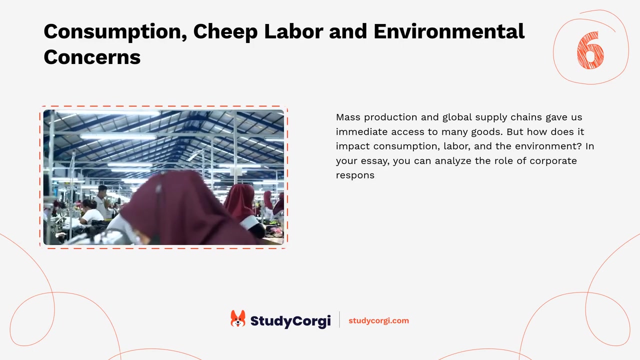 recycling practices and nurturing an environmentally conscious society. Consumption, Cheap Labor and Environmental Concerns. Mass production and global supply chains gave us immediate access to many goods, But how does it impact consumption, labor and the environment? In your essay, you can analyze the role of corporate responsibility and government regulations. 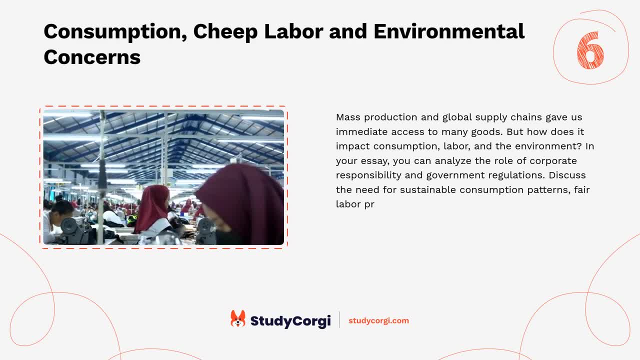 Discuss the need for sustainable consumption practices. In your essay, you can analyze the role of corporate responsibility and government regulations. Discuss the need for sustainable consumption practices. Discuss the need for sustainable consumption practices, Fair labor practices and eco-friendly manufacturing processes to mitigate the 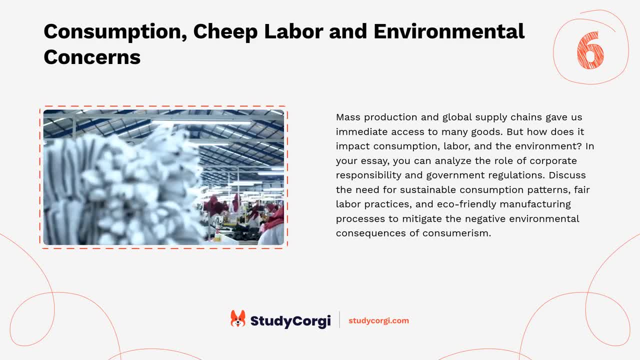 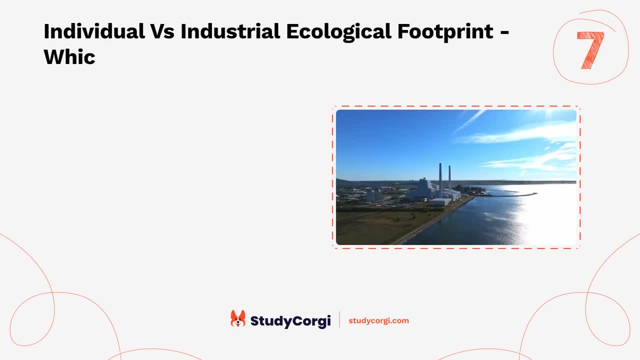 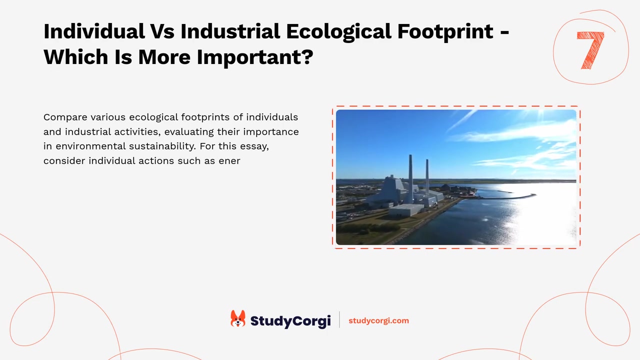 negative environmental consequences of consumerism. Individual versus industrial ecological footprint. which is more important? Compare various ecological footprints of individuals and industrial activities, evaluating their importance in environmental sustainability. For this essay, consider individual actions such as energy consumption, transportation choices and waste generation.